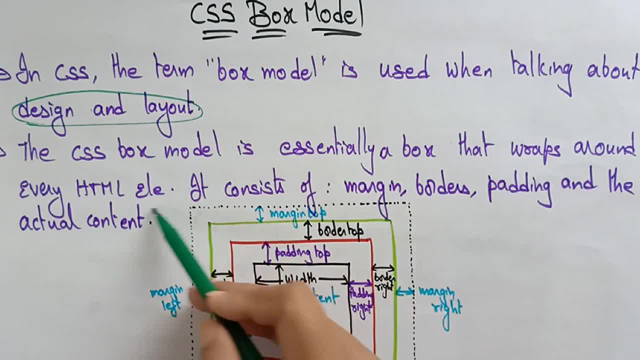 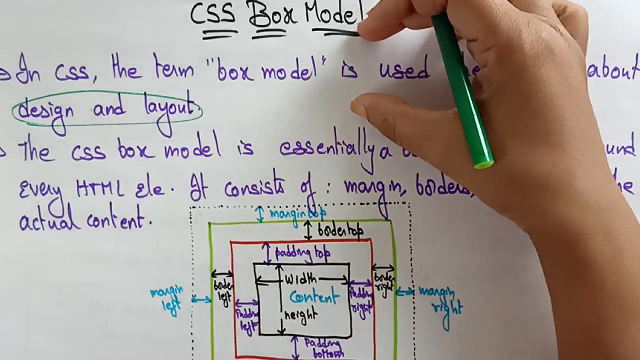 box model is essentially a box that wraps around every HTML element. So this box element is going to wrap, or whatever, the element that you are using in the HTML program HTML. you are using so many tags, the body image, everything, so that everything can be wraps in the box model. It consists of the CSS box model consists of margins, borders, padding and actual 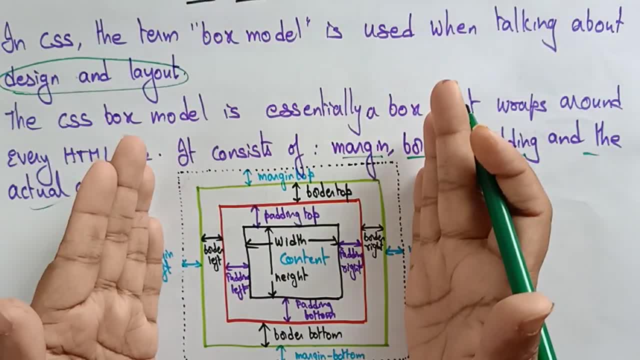 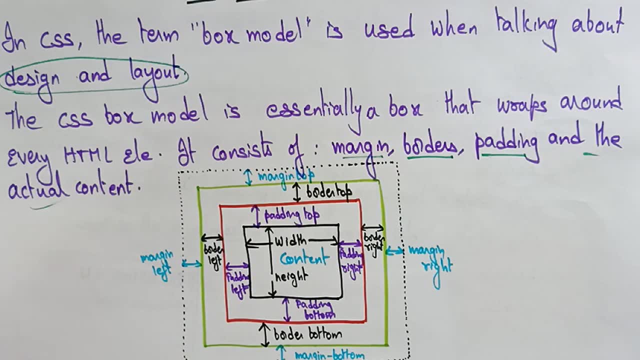 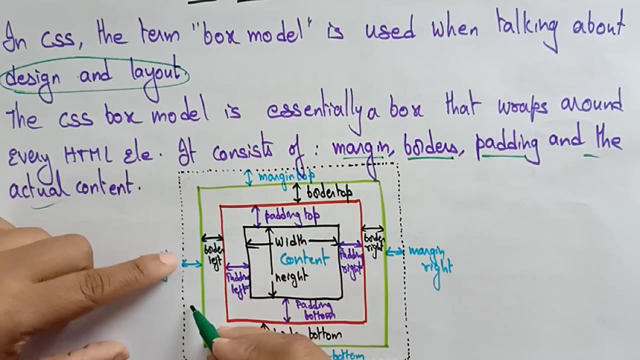 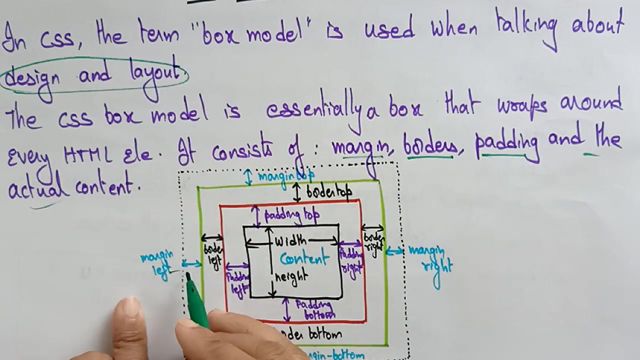 content. So see here, this is diagram. Let us take this is a web page. Okay, the complete web page will be divided into these types. Okay, with margins, borders, paddings and contents. Let's see. The outer one is the. you call it as a margin. Okay, so this is a. this is one margin is the transparent one. It gives us space. If you want to get the space from the left side, left margin, right side, right margin, top margin, bottom margin And after that. 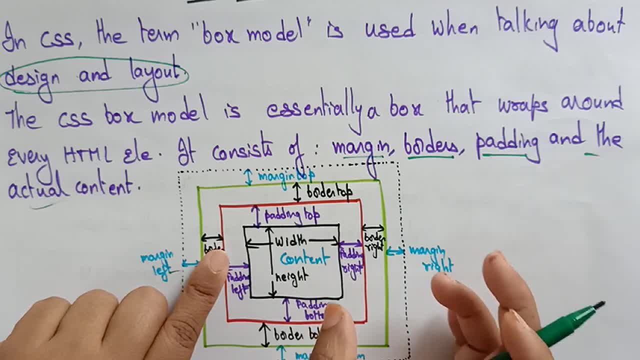 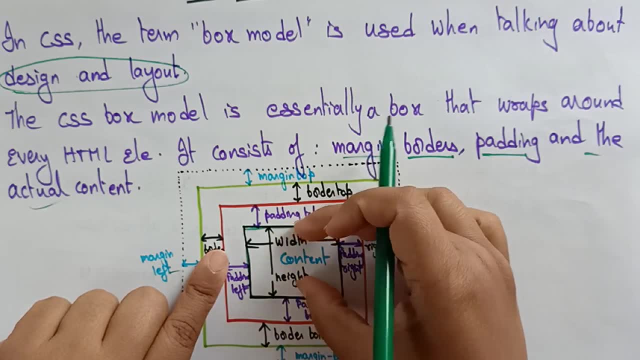 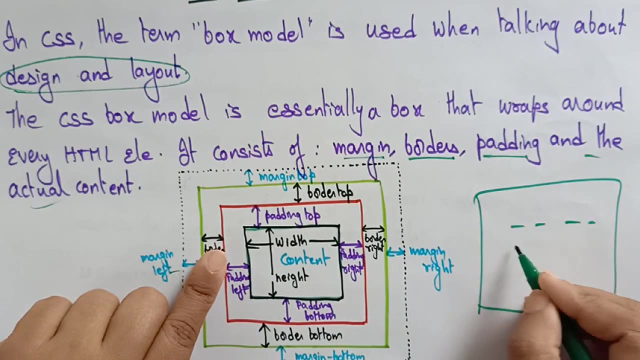 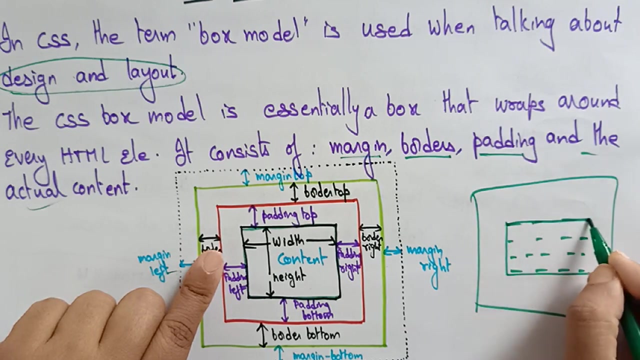 so first starts with the middle, whatever the content that you want to be displayed. suppose the content is present in the web page in the middle, Okay, so based on the height of the content and the width of the content, that content will be I want to appear. I want to print that message in the middle of the web page. So by using this CSS box model, I can print this content in the middle of my web page with all the alignments, with the spaces, with the margins borders. 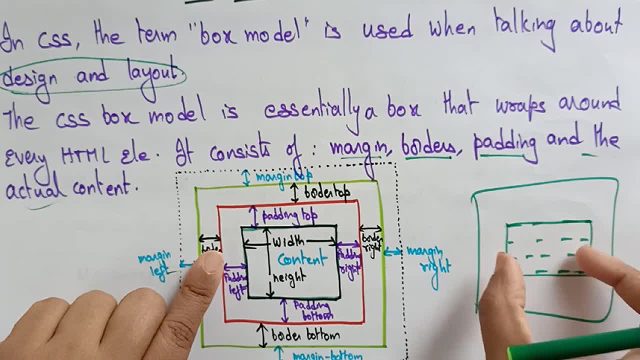 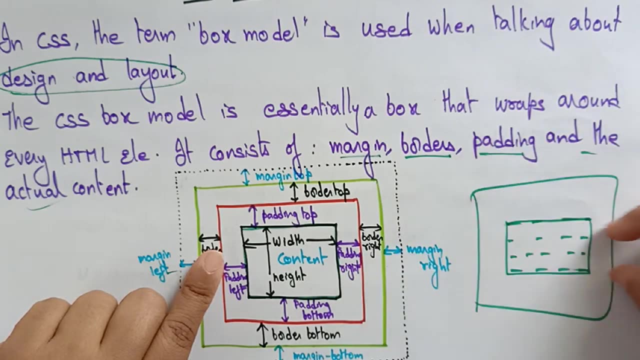 borders, paddings, everything. the text will be appeared in the middle, like, just like css box model. this is a css box model. how it is possible? okay, how my width and the height of the content will be appeared exactly like this. okay, in whatever the format, in the above or below, in the left or 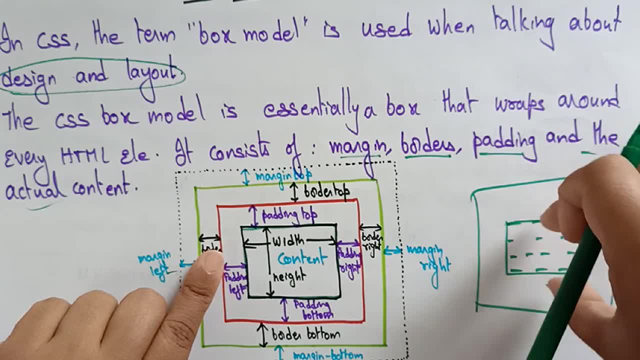 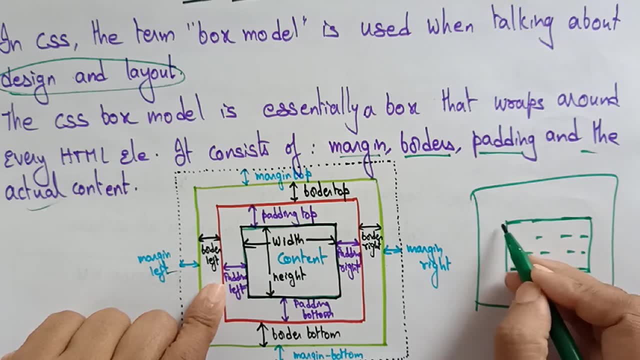 right. so wherever you want, you can print this box. so how it is possible. so first is: whatever the message that you are printing, that message a padding should be there, okay. a padding top, padding left, padding bottom and padding right- okay, so padding is also a transparent. it's just. 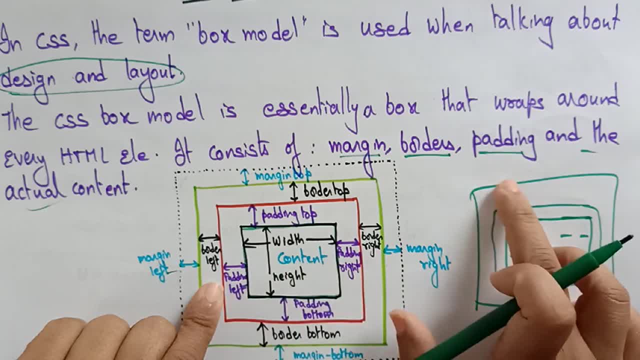 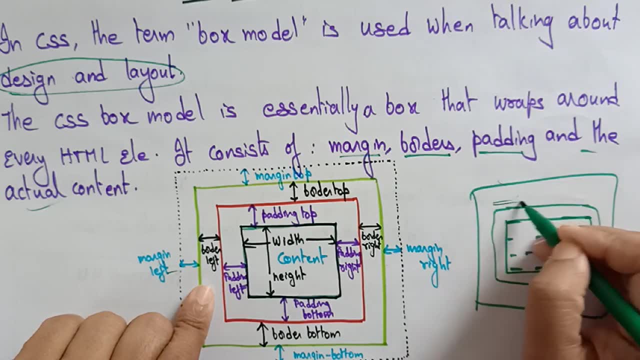 give a space between the borders and the content, between the borders and the content. it's just give a space. that is a padding. next, after padding, you if you want to print some border, like bold or something, the border size, the width of the border, height of the board, everything. 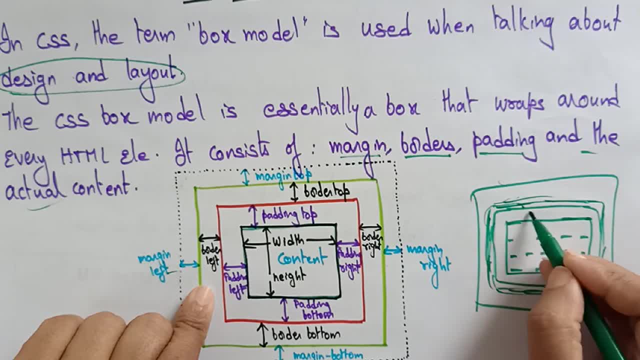 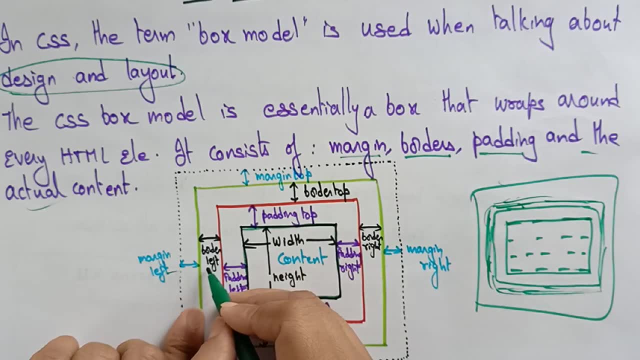 okay, if you want so, here the message will be there and this will be the padding space and here the border you can print: border top, border right, border bottom and border left. after that, again, the transparent margin will be appeared. so this is a css box model. so in the middle the content. 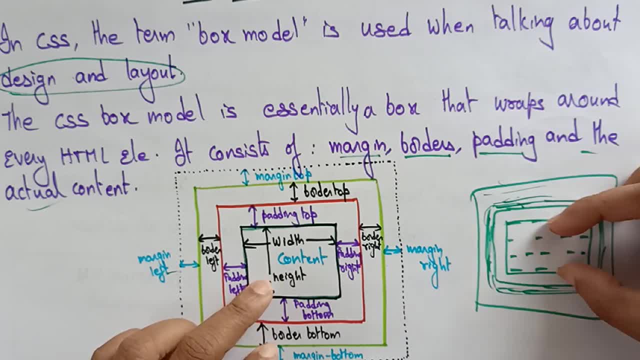 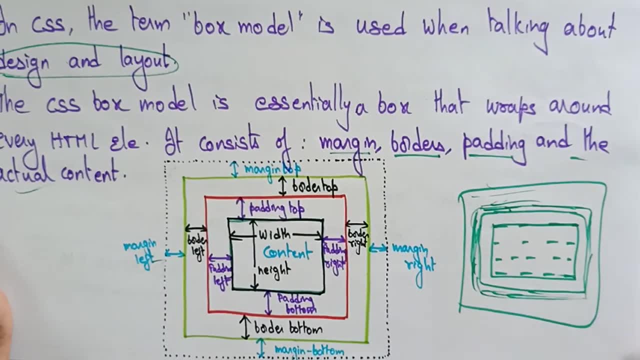 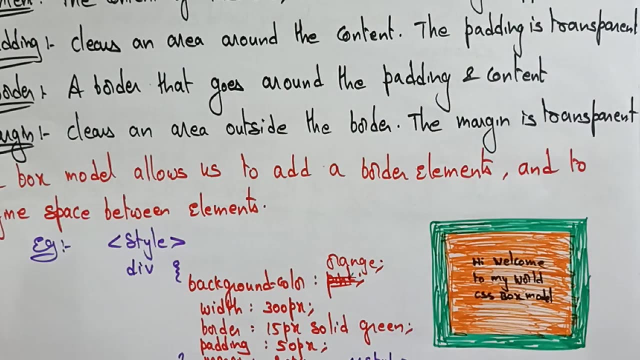 will be there, based on the height of the content and the width of the content. that content will be present exactly in the box model with the help of this padding border and the matching okay, so okay. first, about the css box model. let me explain you with an example, so, before going to know, uh, deal. 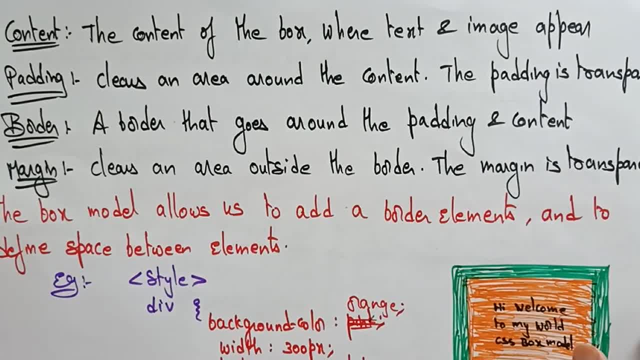 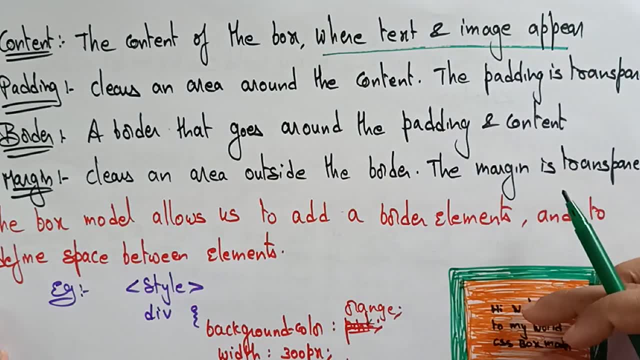 with the example, i want to explain what the content consisting of, what padding border and the margin- content, the content of the box where the text and image appears. so where that that is a place where exactly the text and image will be appeared. so here, this is a content in this way. 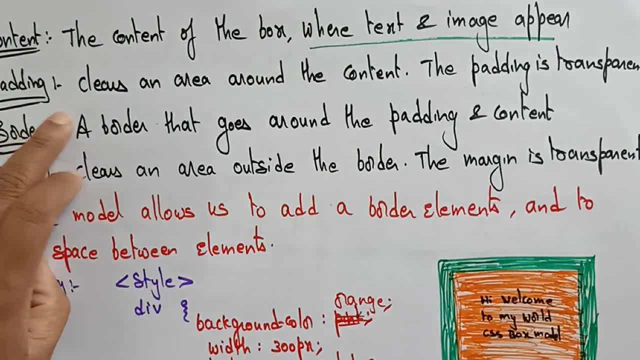 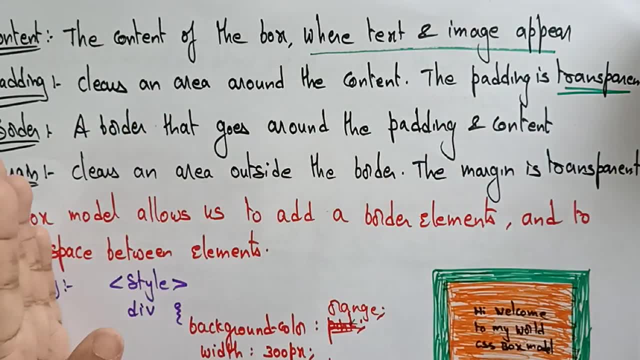 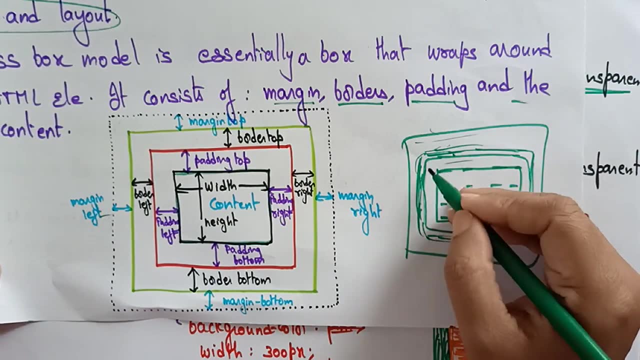 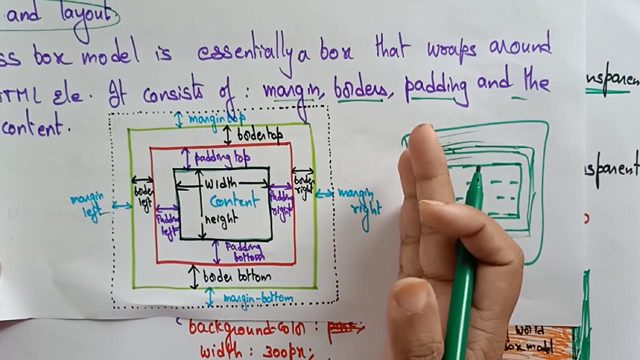 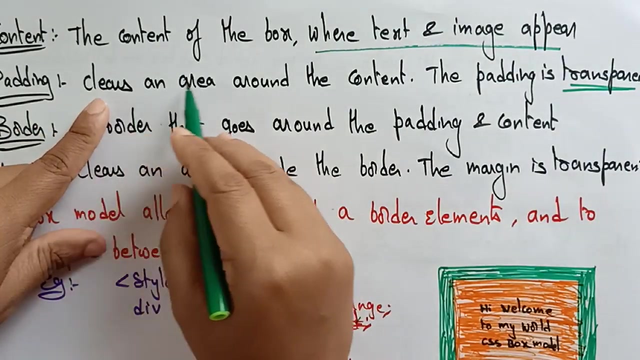 the text and image will be appeared. that is a content padding. it clears an area around the content. the padding will be there and the padding will be there. and the padding will be there. and the padding here is a transparent, so it's just make it clearer. uh, it want to make something transparent here, so what? 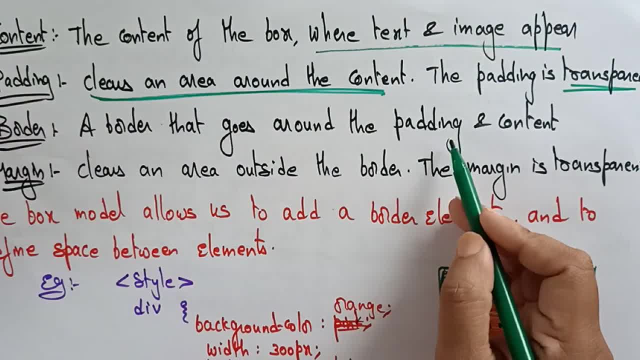 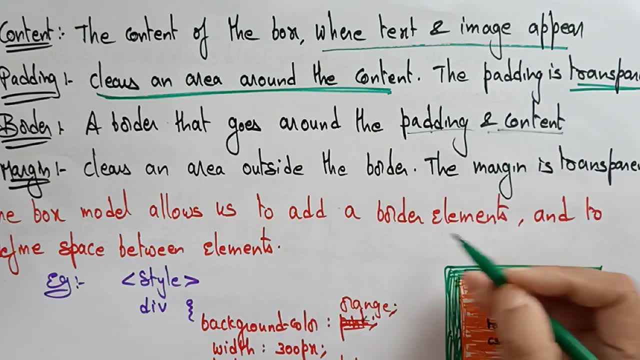 so that no one will enter into this field. okay, you can't enter into this field so that it should look and the padding is transparent border, a border that goes around the padding and content. so it just displays a border and margin. it clears an area outside the border. so in outside the border. 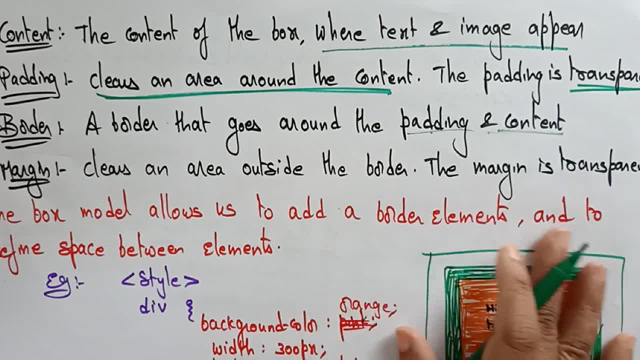 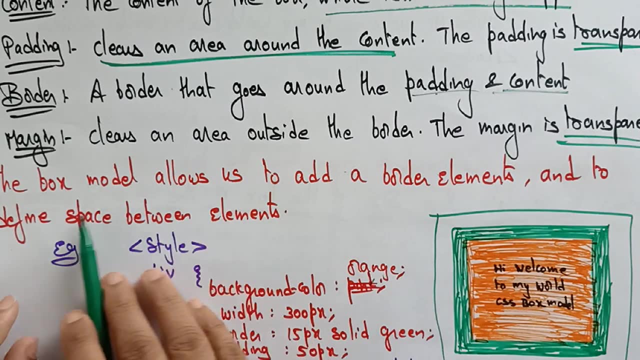 also it clears the uh just like a padding. the margin also clears. but if the margin is outside the border, the margin is also a transparent. so let's see an example to know this box model, the more the one thing that you have to remember that the box model allows us to add. 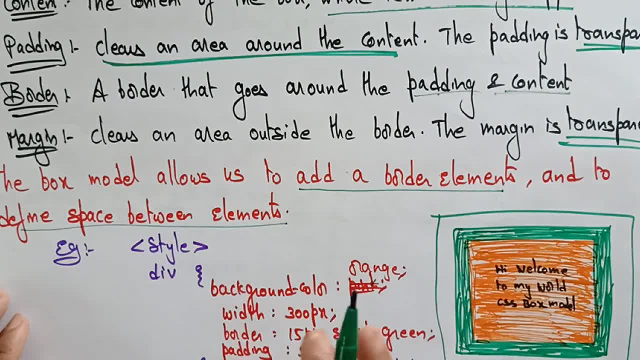 a border elements and to define a space between the elements. so it allows to add a border elements. so these are the border elements. means what type of border you want. you want the bold border, you want the different color border, you want the design border, whatever the so it allows us to. 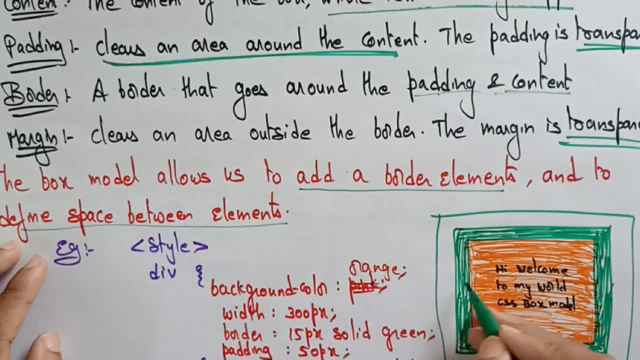 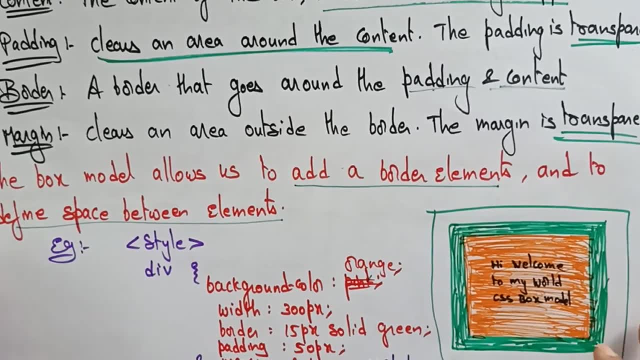 add a border elements and to define a space between the elements. how much space i need to be present in between the borders and the margins and the padding, like that? okay, so let's see the program. so here the style tag. so within the style tag i'm, i'm using the div as a selector. 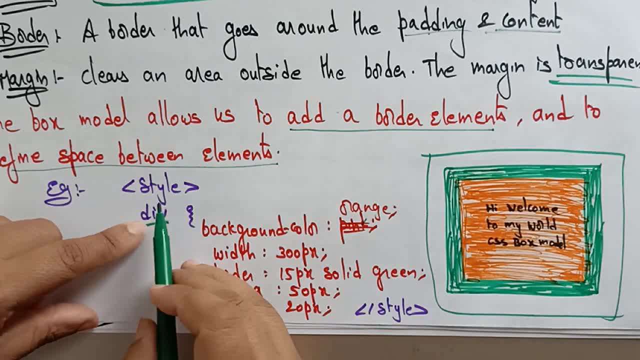 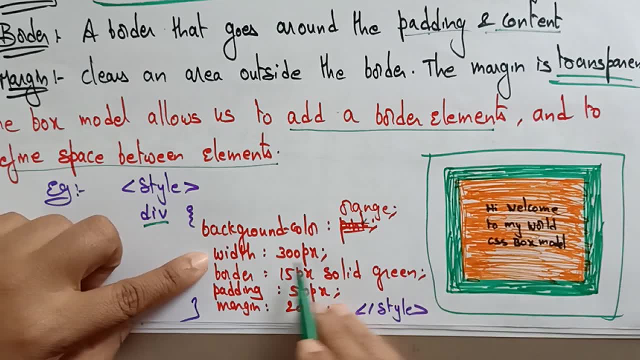 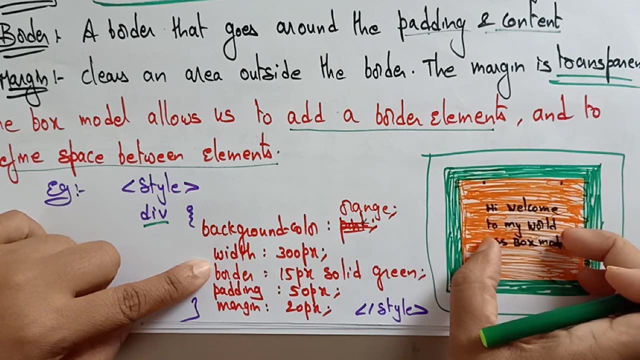 so i'll use this. i will call this div in my body section: okay, style div. so the background color is the orange, so everything the background color should be the orange and the width of the content is the 300 pixels. so from here to here, the width of the pixel is the 300. 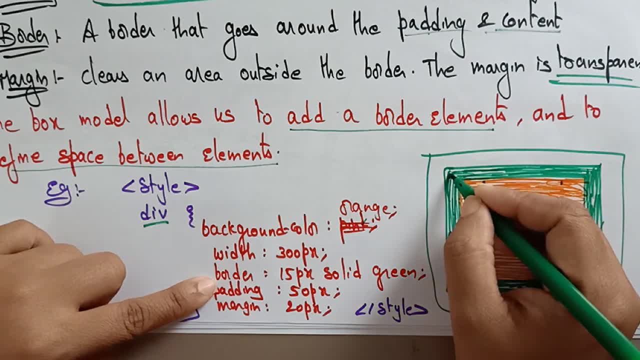 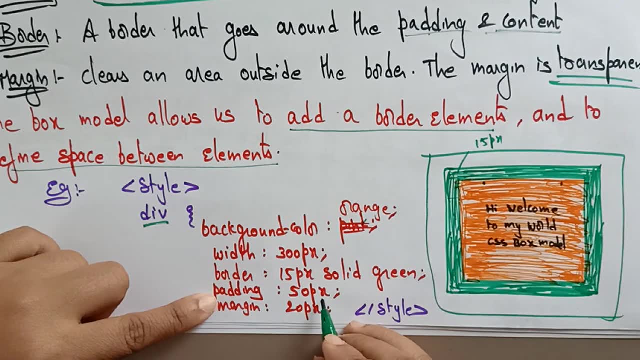 okay, and the border is the 15 pixels solid green. so this is a border of 15 pixels. this is 15 pixels solid green and the padding is 50 pixels means in between this content, in between this content and between the border. so the space you are seeing here, okay, so this space is the 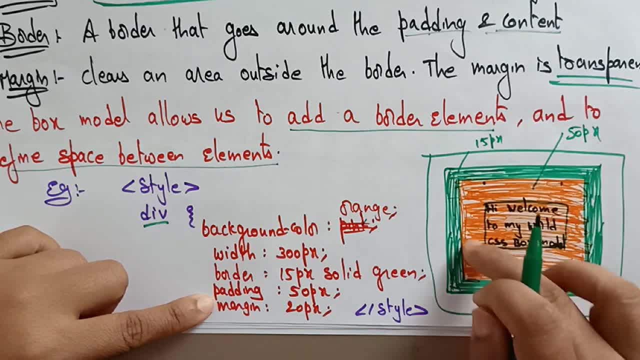 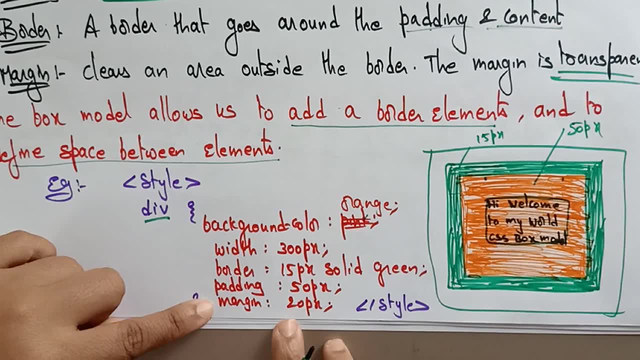 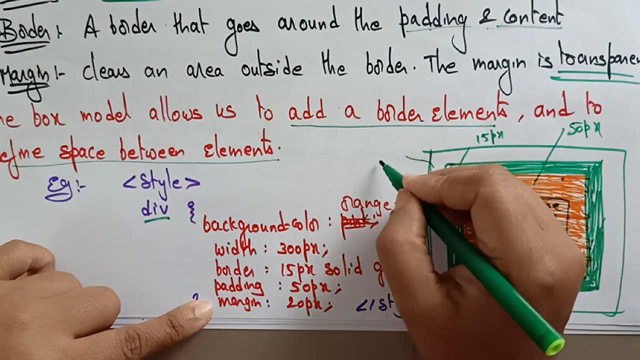 padding. it's a 50 pixels, so this is all the complete transparent space between the border and the content. this is a padding that is a 50 pixels and the margin is 20 pixels. there is a margin that is a transparent, so this is my web page and this is a margin of 20 pixels, which is also a transparent. 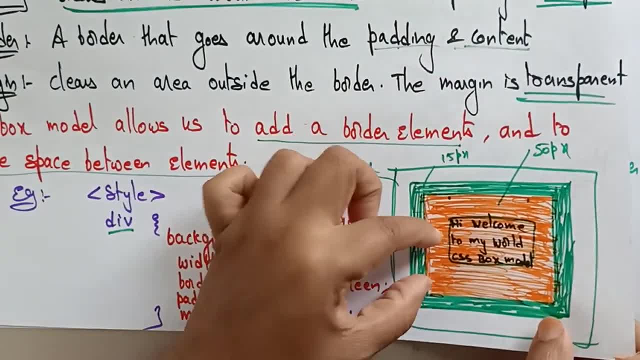 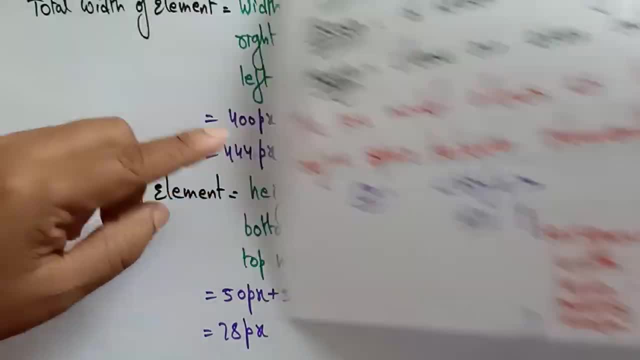 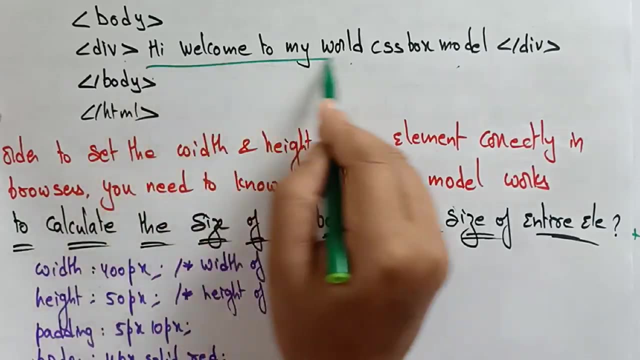 okay, so how i get this message? it this is my output. how i get this. see here the body div. i'm just calling whatever the selector i have using this div and the message is: hi, welcome to my world css box model and the body close. so this message is appearing in the box model. so in this way, 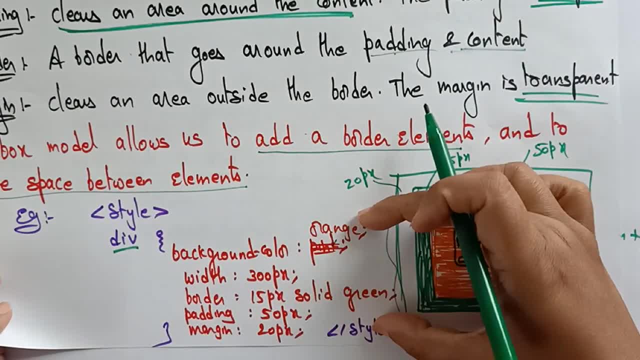 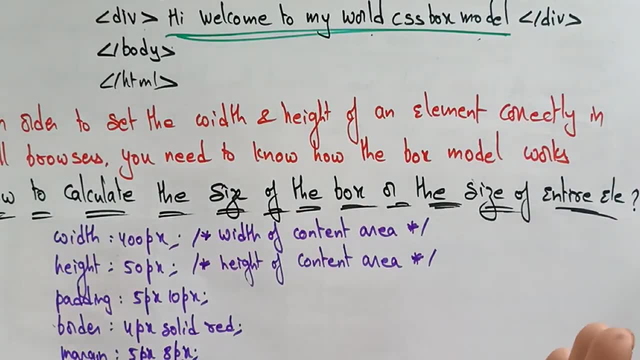 it will be appeared how with the help of all this content. okay, so in order to set the width and the height of an element correctly in all browsers, you need to know how the box model works. okay, by default you can't set because different browsers having the different uh window sites. okay, so in 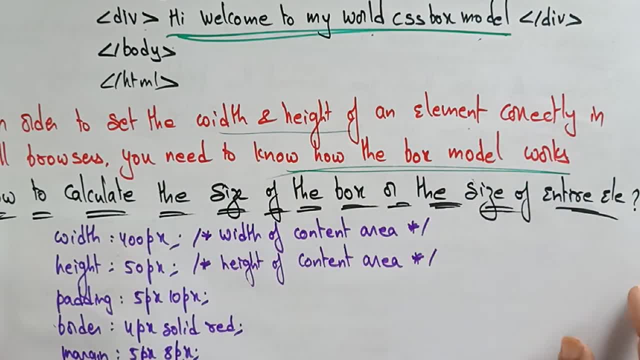 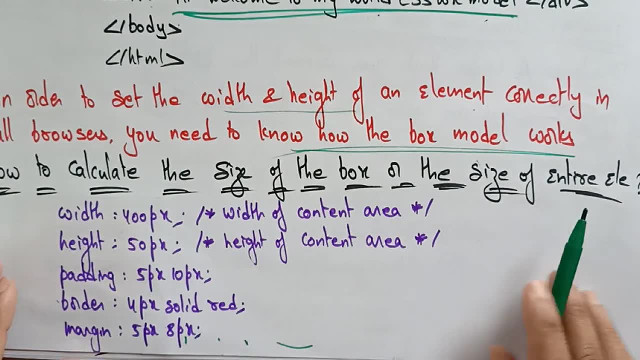 order to set the width and the height of an element correctly in all browsers, you need to know this box model works. now let's see how you, how we, are going to calculate the size of the box or the size of the entire element that we are using. okay, you need to calculate the box of the size. 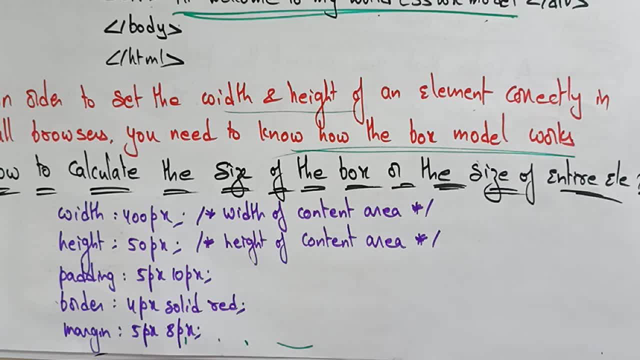 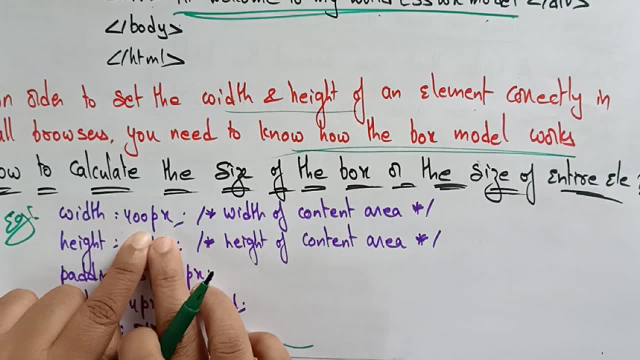 based on the box of the size only. the matter will be appeared clearly on different browsers, so let's take one example here: the width. i am taking 400 pixels. this width means the width of the content area, whatever the message that is there. there, the width should be this from starting to here. this is the 400 pixels width and the height. 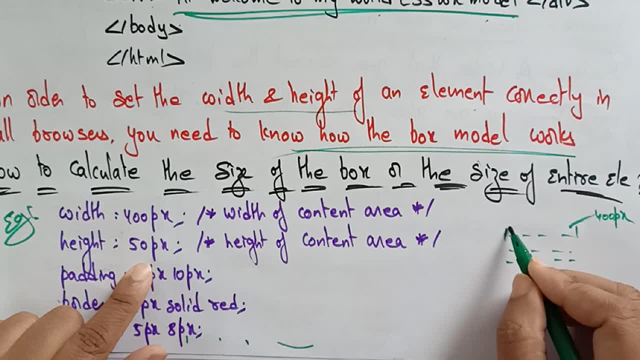 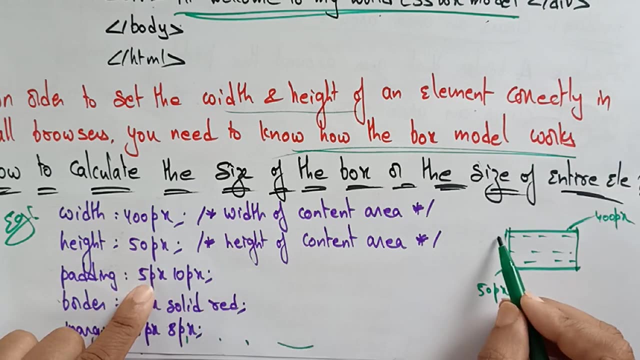 of this is 50 pixels means this is the height, so I am taking it as a 50 pixels. so this is the width is a 400 pixels and the height is 50 pixels. so like this, the message has to be appeared and the padding is 5 pixels means the space between the borders and the content is the 5 pixels and 10. 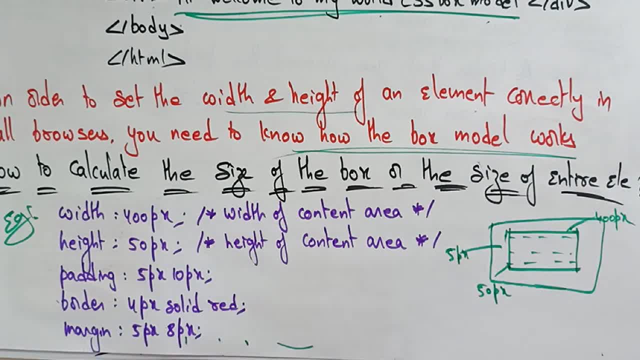 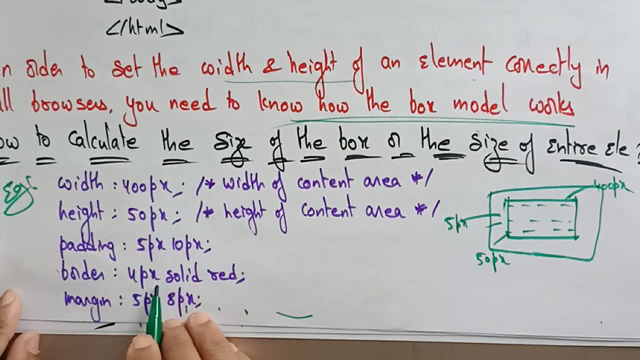 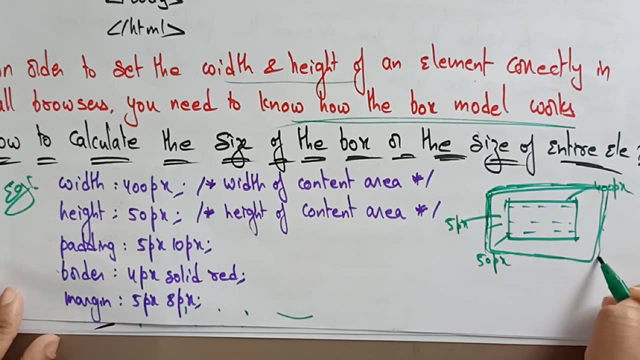 pixels means the width and top and the bottom, sorry, left, right, so the left and right, top and bottom. 5 pixels and 10 pixels. border is a 4 pixels solid red, so the border should be the solid red. I have to be printed the solid red. that border width is a 4 pixels and the margin is 5 pixels, 8 pixels. 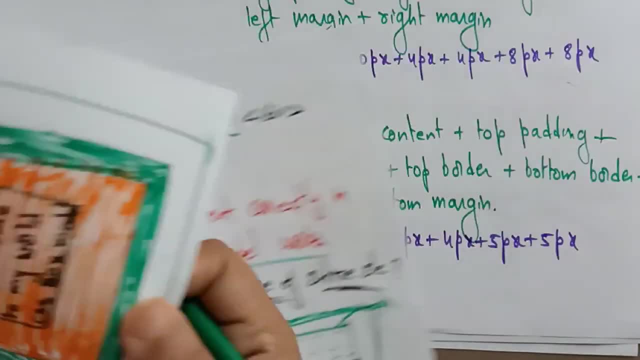 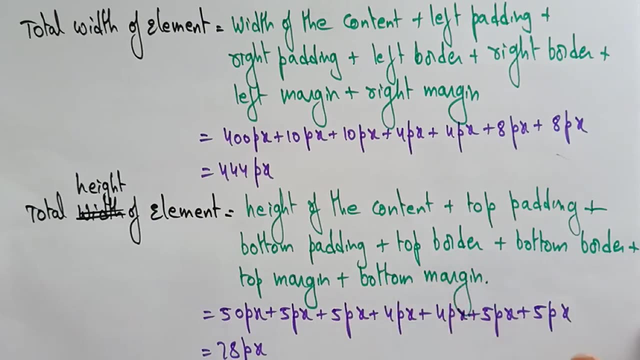 now let's see how I am going to calculate the height and width of the: the total width of the element and total height of the element. so I am going to calculate the height and width of the height of the element. Let's see here, With the help of this formula, the total width of the. 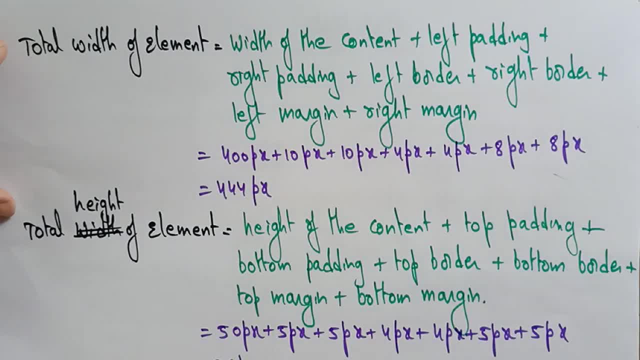 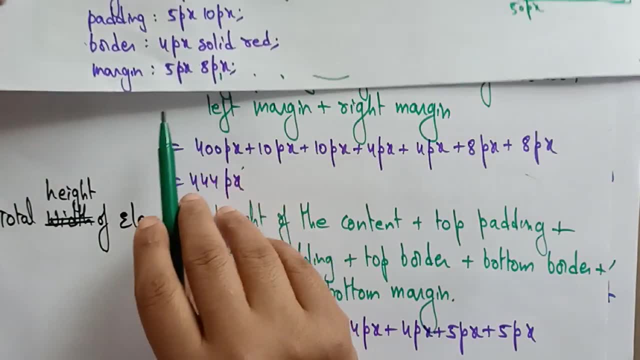 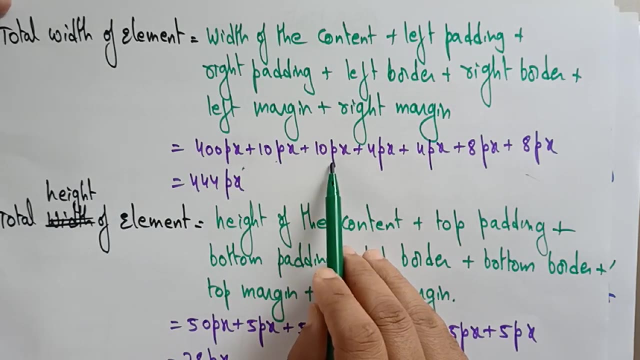 element formula is the width of the content. So what is the width of the content? The width of the content is 400 pixels and the left padding- the padding is 5 pixels and 10 pixels. okay. The left padding is 10 pixels, 10 pixels. right padding is 10 pixels. okay, And so this is about. 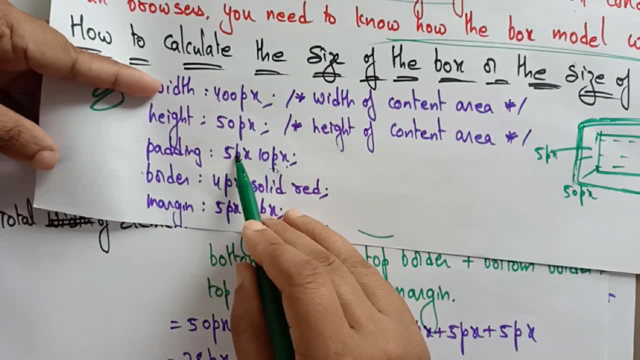 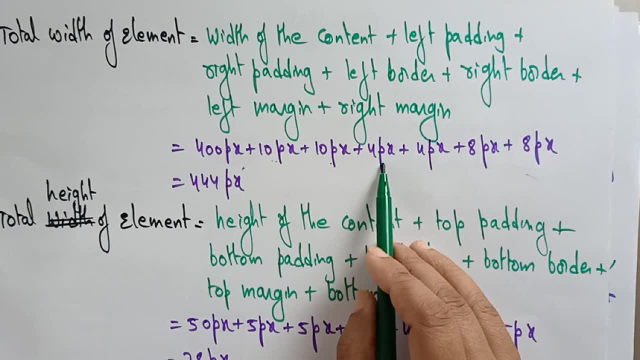 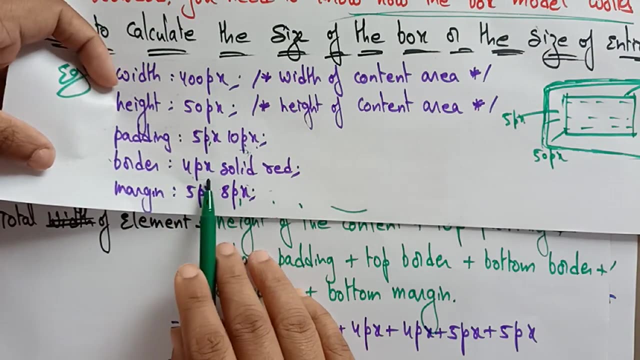 left and right and this is about the top and bottom, left and right, top and bottom. So left pixel 10, right padding 10, left border 4 pixels, right border: 4 pixels. So the border they are giving is 4 pixels, solid red. In all the sides there is a border size will be the same, So 4.